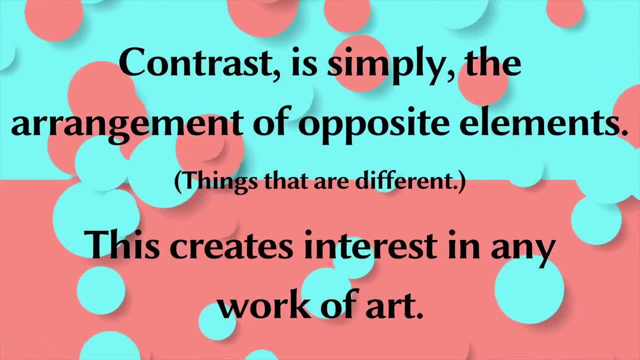 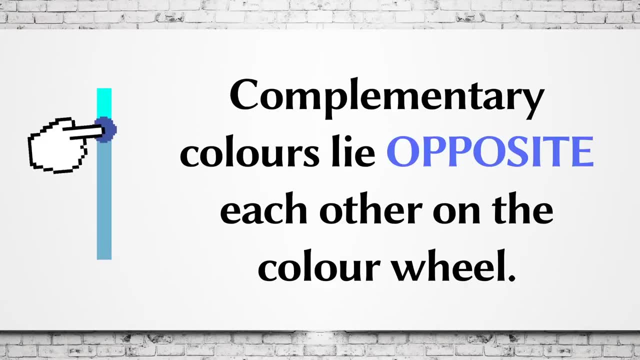 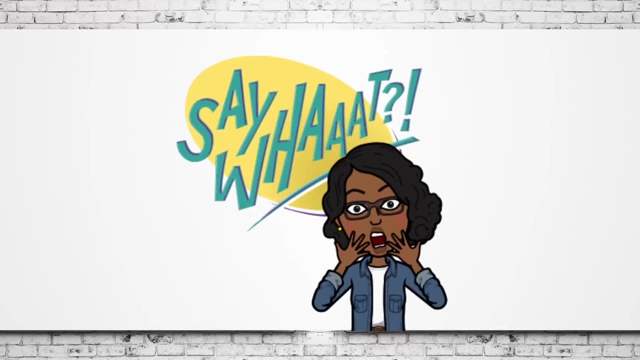 Simply the arrangement of opposite elements, things that are different. This creates interest in any work of art. Complementary colors lie opposite each other on the color wheel. Today is Opposites Day. What are you wearing today? What am I going to do? I completely forgot that today is Opposites Day. 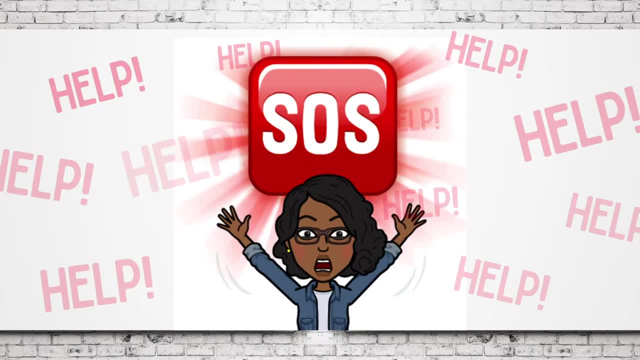 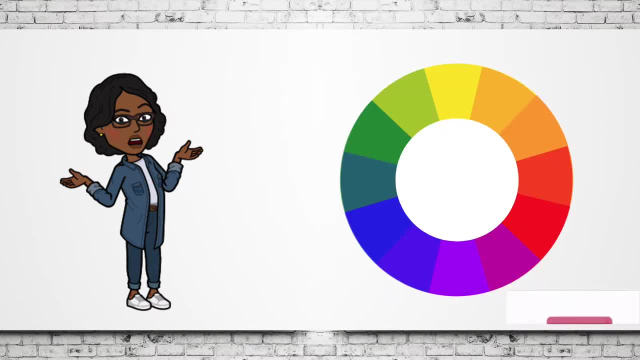 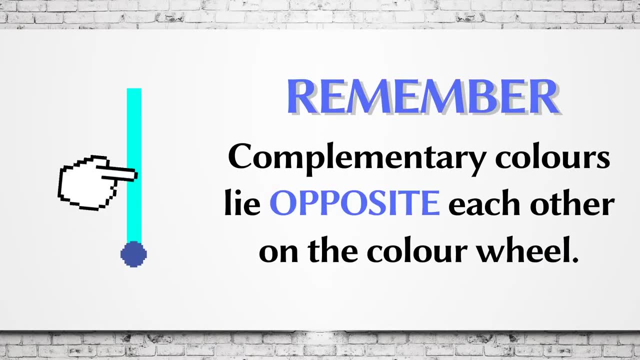 I really need your help, everyone. Can you please help me find the perfect outfit to wear for Opposites Day? What should I wear today? I really like the color yellow, But what is the complement of yellow? Remember, complementary colors lie opposite each other on the color wheel. 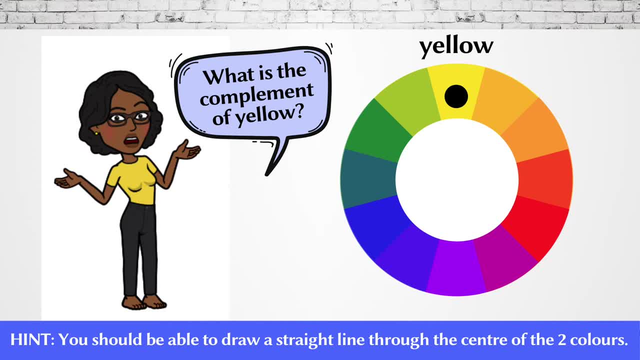 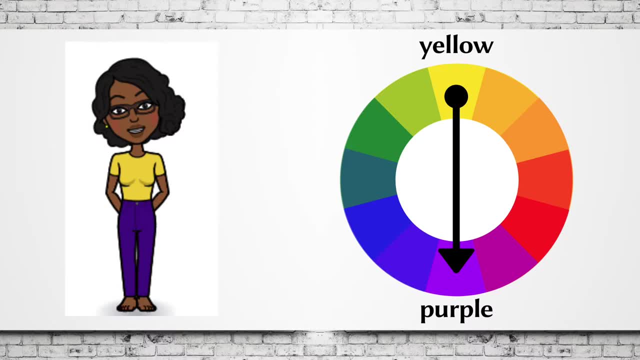 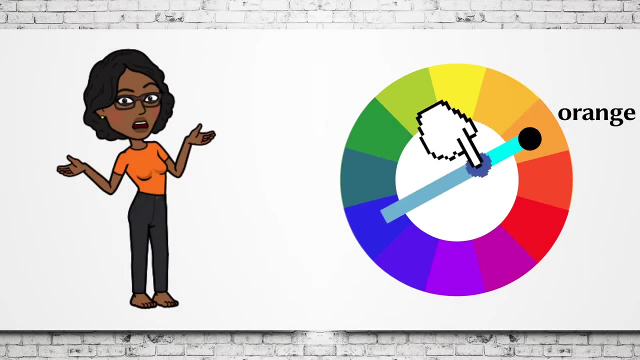 Here's a hint: You should be able to draw a straight line through the center of the two colors, Just like this. So the complement of yellow is purple. Now what if I would like to wear an orange t-shirt? Begin by drawing a straight line through the color orange. 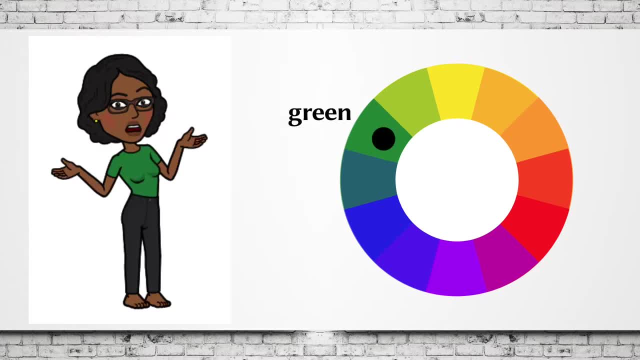 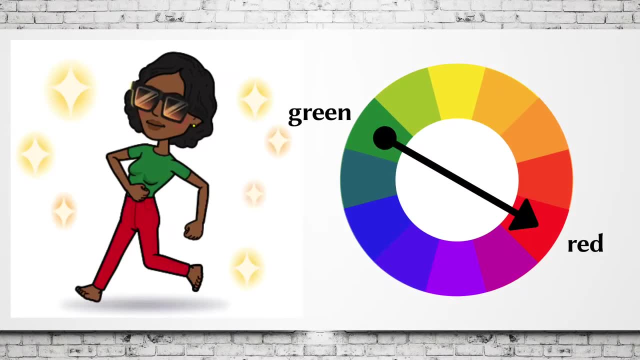 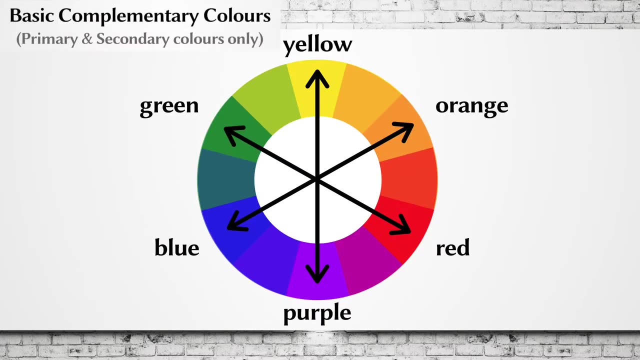 That's right. Blue is the complement of orange. Green is my favorite color. What is the complement of green? Yes, red is the complement of green. These are the basic complementary colors, using the primary and secondary colors only. Here are the other pairs of complementary colors. 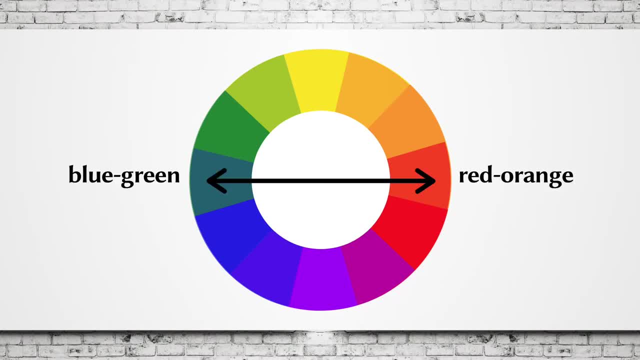 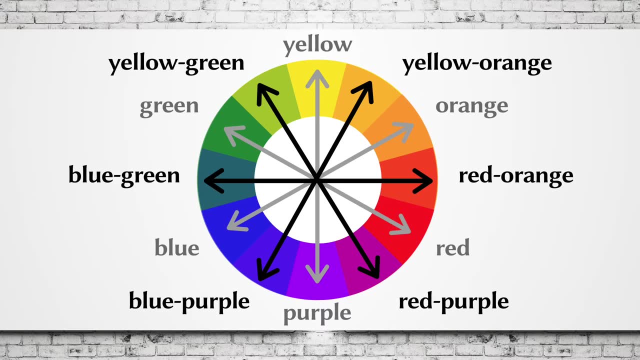 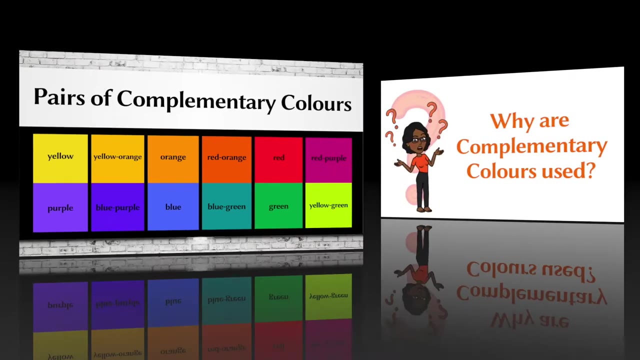 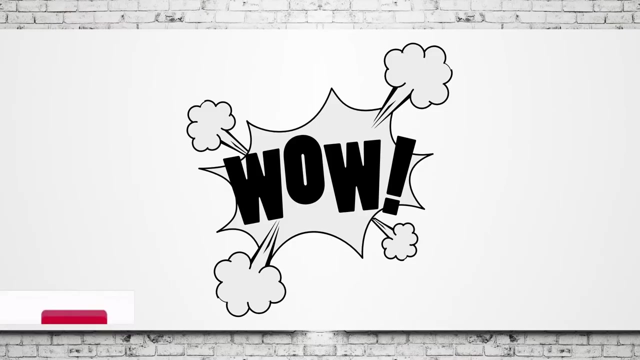 Yellow, green and red purple. Blue green and red orange. Yellow orange and blue purple. Now let's take a look at the pairs of complementary colors. When complementary colors are placed next to each other, they appear brighter. 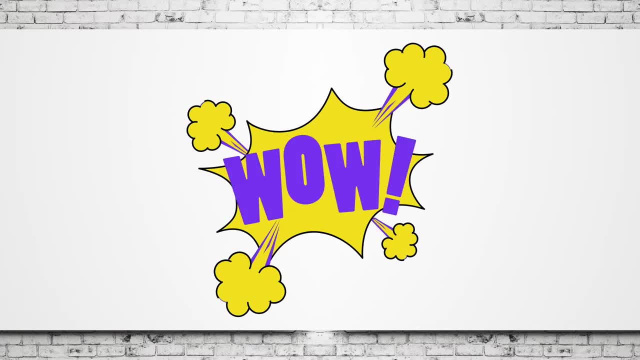 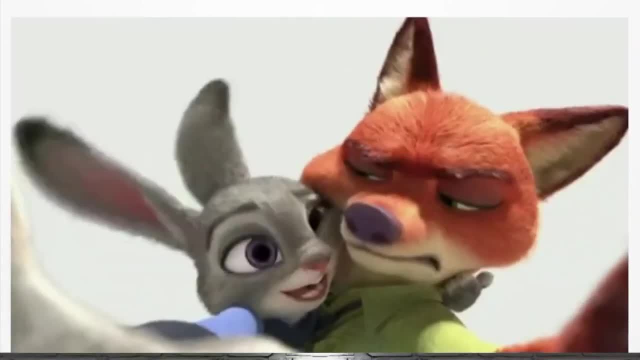 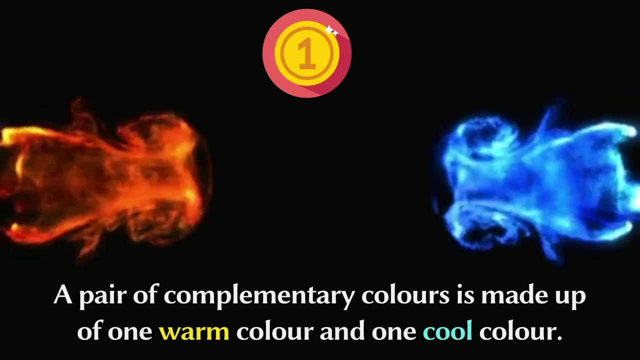 When complementary colors are placed next to each other, they appear brighter. This allows parts of your artwork to stand out, thus grabbing the viewer's attention. In other words, complementary colours behave like best friends. They are better together. Here's how A pair of complementary colours is made up of one warm colour and one cool colour. 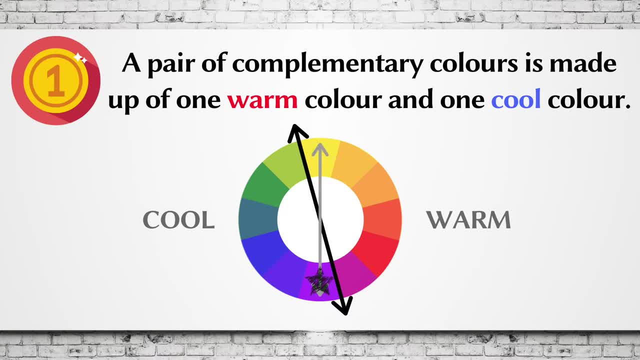 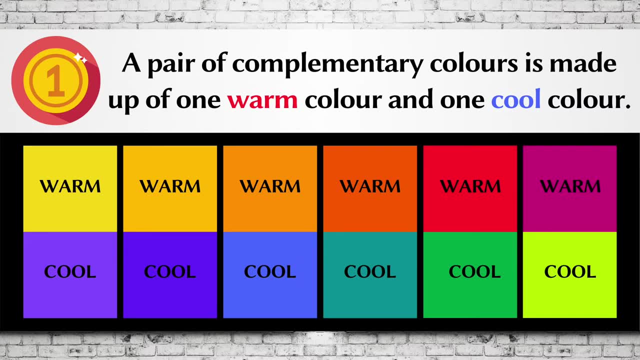 For example, yellow is a warm colour and purple is a cool colour. No matter the pair, one colour will always be warm and the other will be cool. These colours have opposite temperatures. This creates high contrast. Let's take a look at the basic. 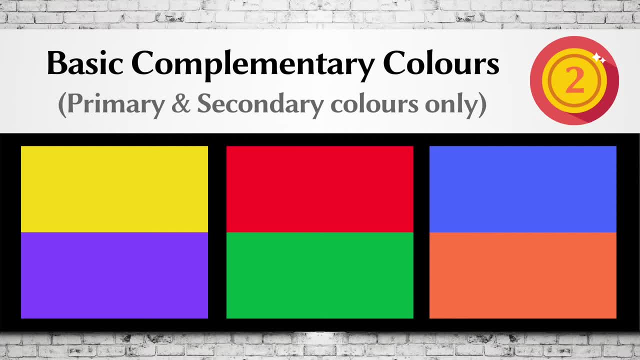 complementary colours. These pairs of colours have the greatest level of contrast. Not only are they thermal opposites, they are also opposites based on how they are mixed. Red is a primary colour and green is a secondary colour. There is no red in the colour green. 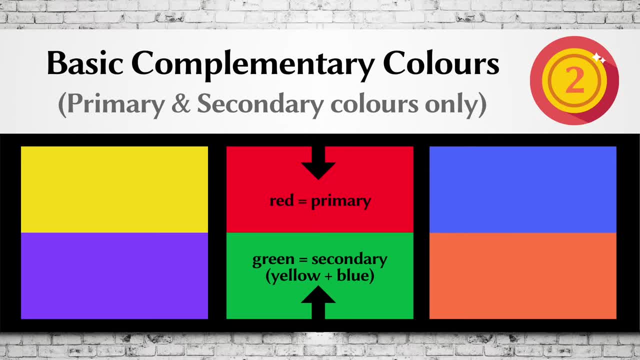 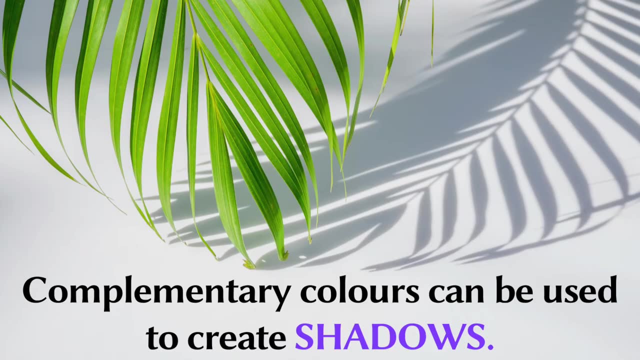 Only yellow and blue. This means that when they are placed next to each other, red does not have to compete with another red-based colour like purple or orange. The same thing applies to the other pairs of basic complementary colours. Complementary colours can be used to create shadows Using a colour's complementary colour. 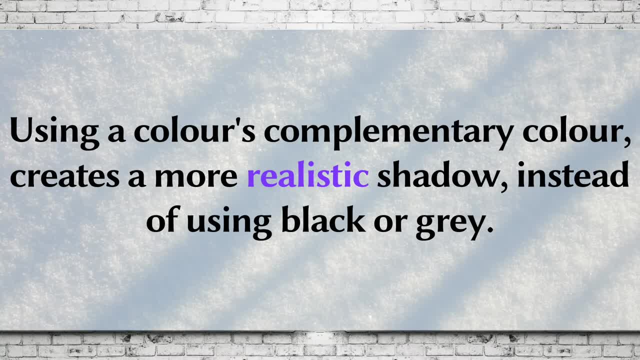 creates a more realistic shadow instead of using black or grey. If you are painting a banana or a long tree, you can use complementary colours to create shadows. If you are painting a banana or a long tree, you can use complementary colours to create shadows. If you are painting a banana or a 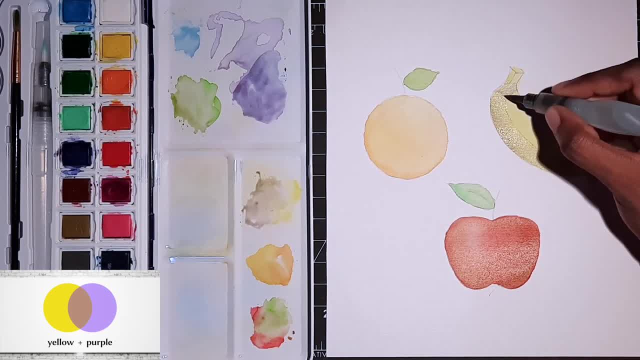 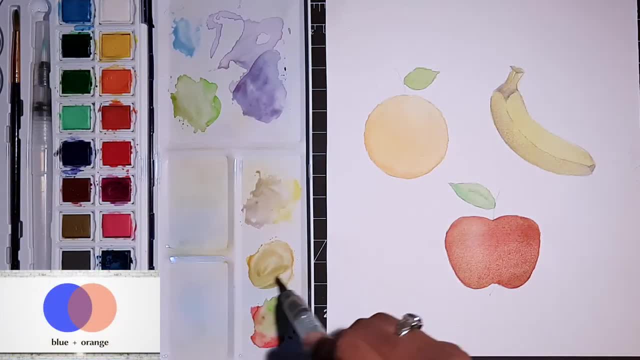 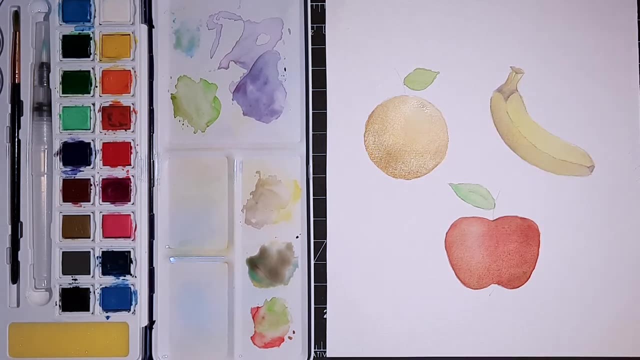 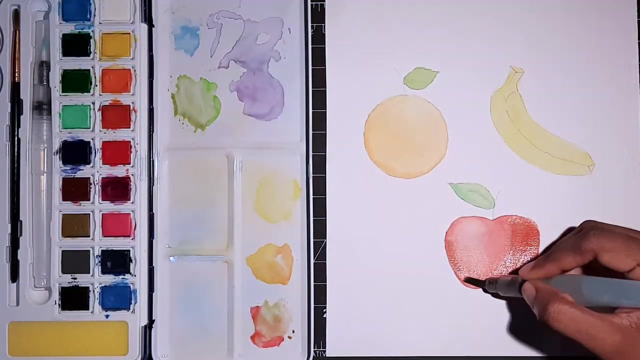 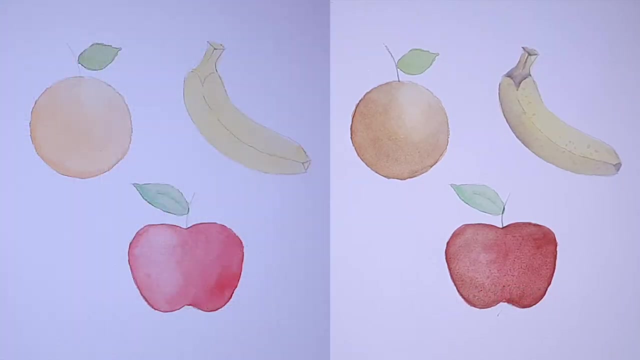 lemon. instead of going straight to the black paint, use a little purple. If you are painting an orange, add some blue, And if you are painting an apple, use some green. Let's look at some artworks where complementary colours have been used. 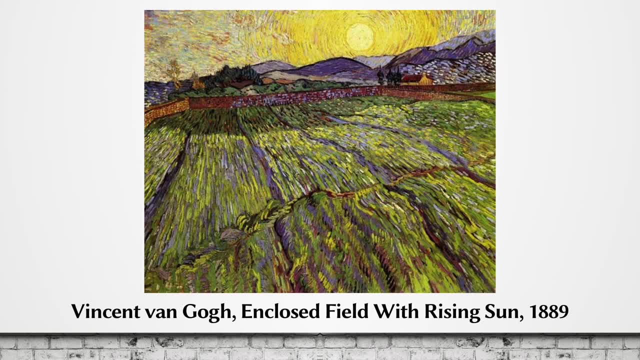 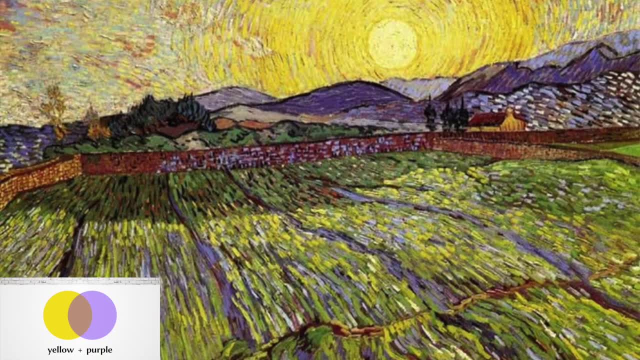 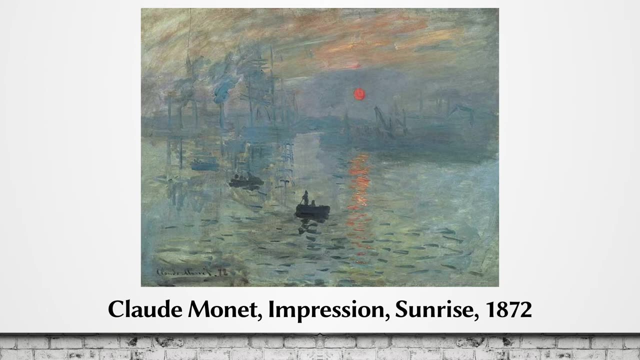 First up, we have a painting by Vincent van. Gogh. What stands out when you look at this picture? The yellow sun and sky pop out from behind the purple mountain range. Next, we have a painting by Claude Monet. What stands out when you look at this picture? 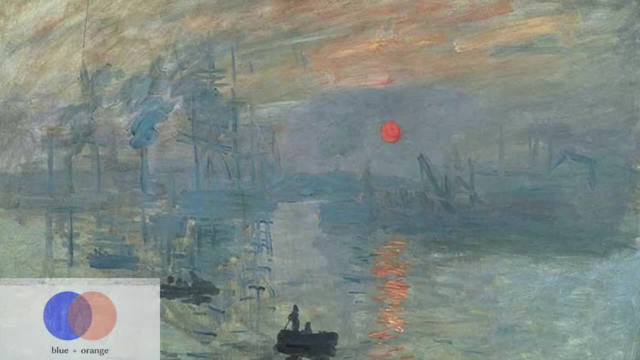 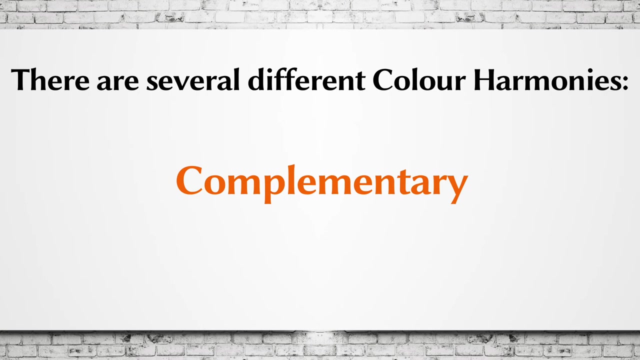 Although it takes up a very small part of the painting. the orange sky, sun and reflection in the water stand out against all the blues of the sky and the sea. And that wraps up our lesson on complementary colours. Let's review the most important parts. Remember complementary colours lie opposite each other. on the colour. 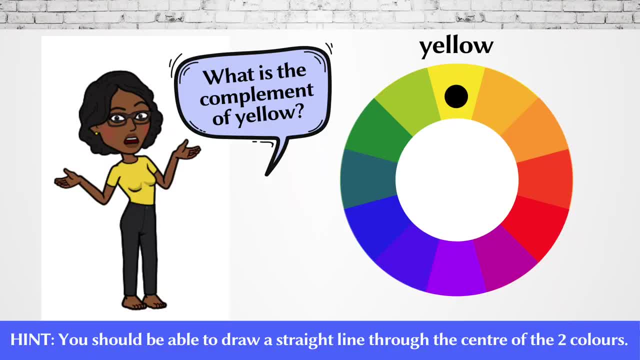 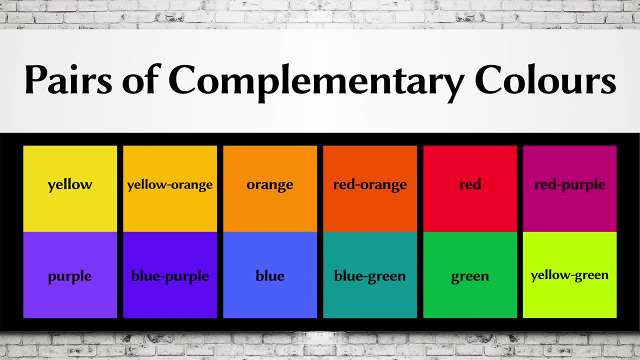 You should be able to draw a straight line through the centre of the two colours, just like this. I hope you learned something new about complementary colours. If you would like to know more about colour theory, you can watch some of my previous videos. 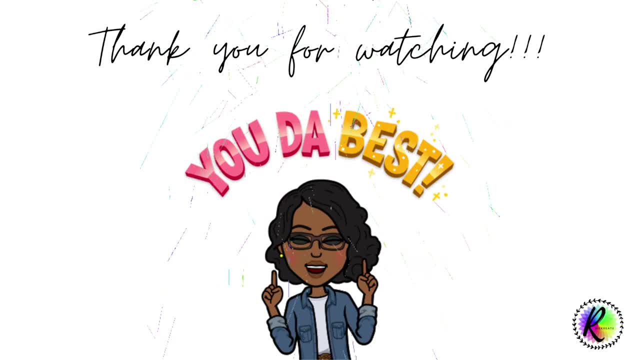 The video links will be in the description box below. Thank you for watching.